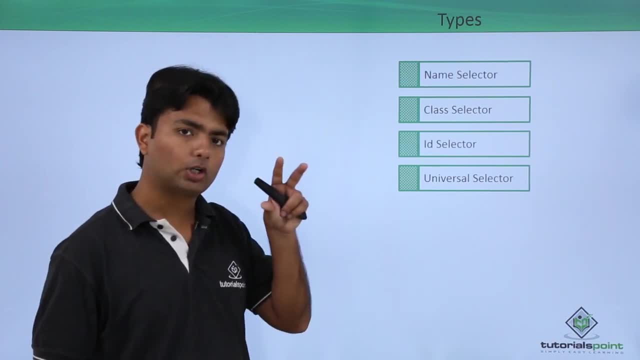 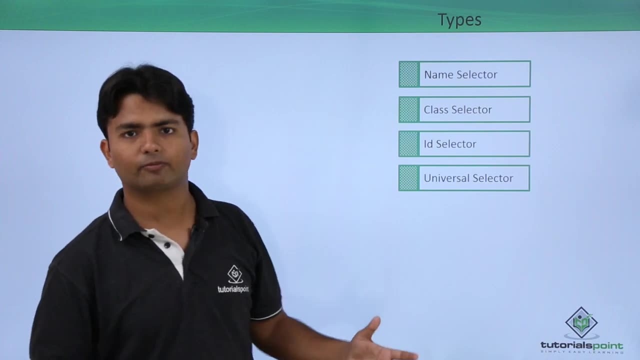 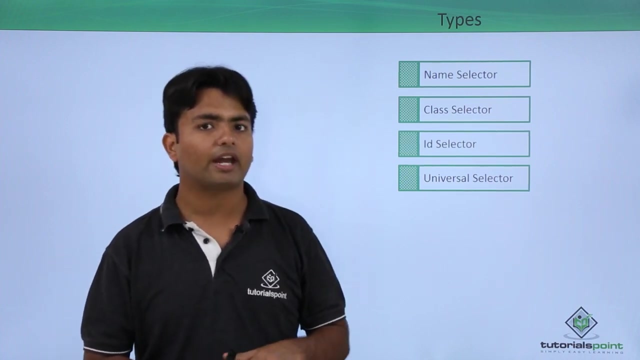 the same value on the same web page. So if for a particular div or something you want to put a style, you can use the id selector, and universal selector is something where you will put the style for the complete DOM. So let's get started with the practical implementation and can see. 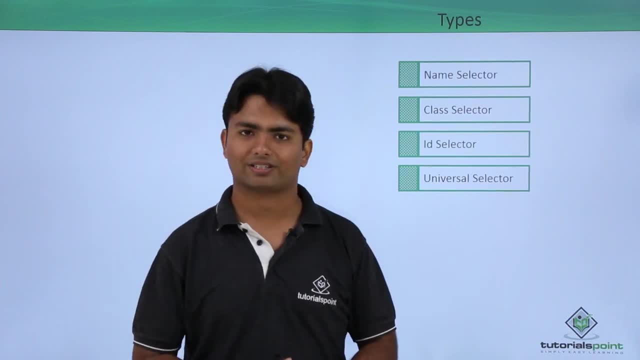 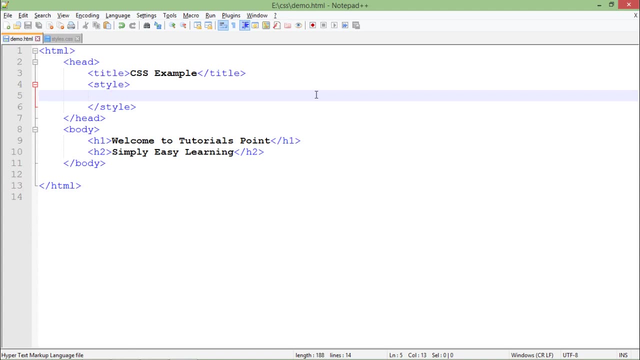 how these different selectors can be implemented. So for starting the implementation of selectors, I will use the embedded style sheet. just to make sure that the style sheet is embedded, You can see the styles and the tags on the same page, so it will be easier for you to understand. 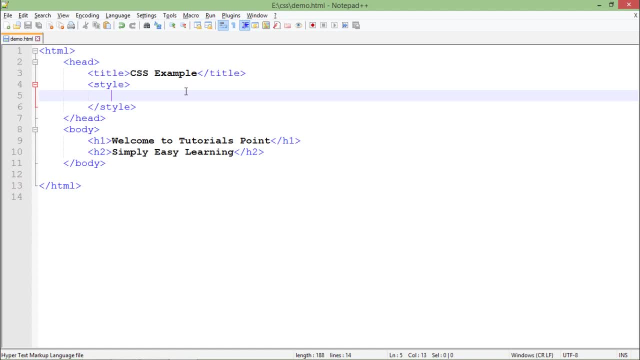 So now what I'll do. I'll start working with the name selector, as we have seen so far in the video that here I can pass any particular name of the element, like h1,, h2, p, paragraph bold b. all right, So such things can be decorated by using the name selector. 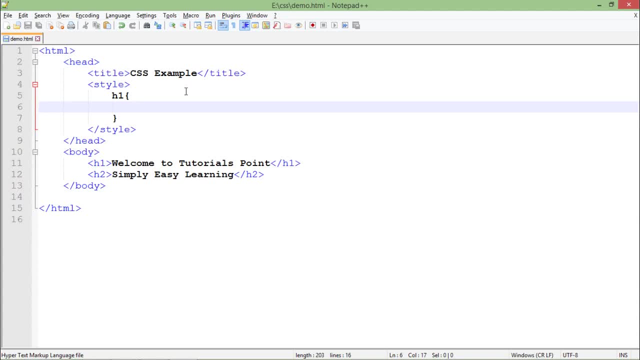 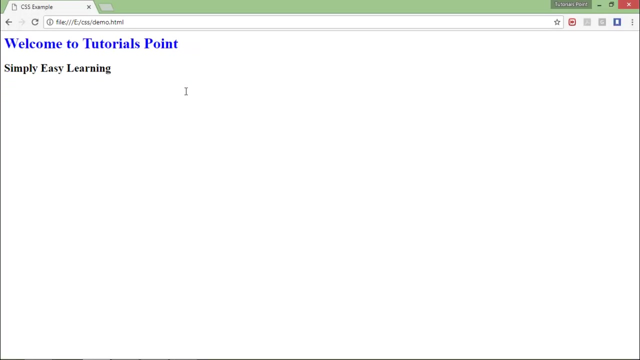 And we will use the name selector in the situation when you want that complete document should get the same styles for all the similar tags. For example here in h1. if I'll say color to blue, then all the h1 of this particular tag will be converted to the blue font. 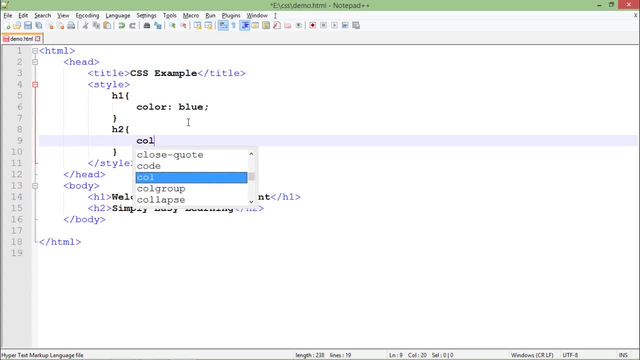 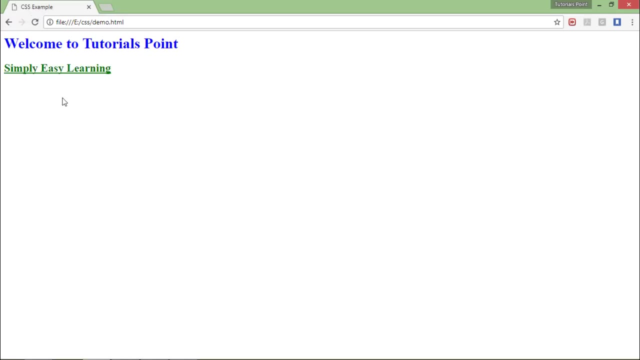 Alright. similarly, if I'll say to to color green and text decoration to underline, so it will be reflected to all the h2 tags. all right, like if I will copy and paste it again, so you will see all the h2 tags, whether I have written anything here or not. all will be. 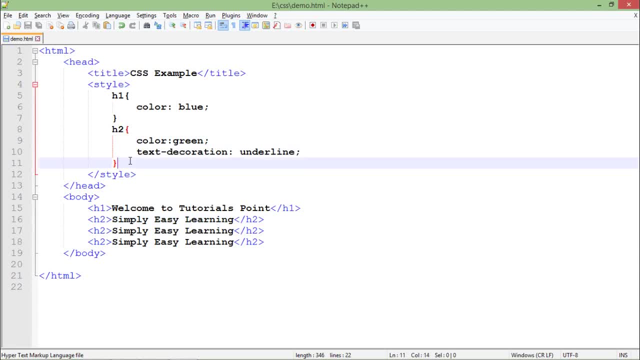 decorated with the same styles. similarly, you can pass the same styles to the multiple elements at the same time. for example, I have a couple of tags like for bold tag and for the italics tag. I want them to be degraded with the underlines. what I will do? I will just put the text decoration underline here. 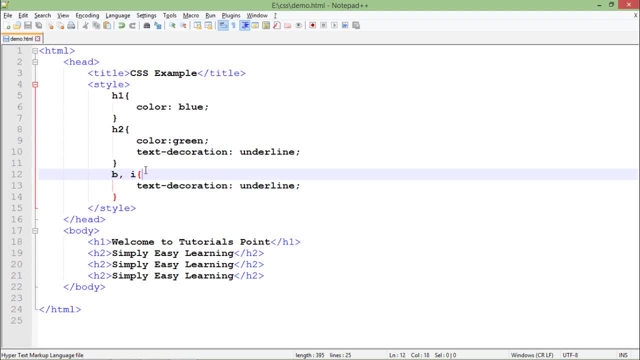 and you can see here B comma I. that means for the bold as well as for the italics. I will decorate the text with the underline, so let's see how it will be looking like. so here I'll put a bold tag like: this is bold. I'll close the bold tag, I'll break the line and 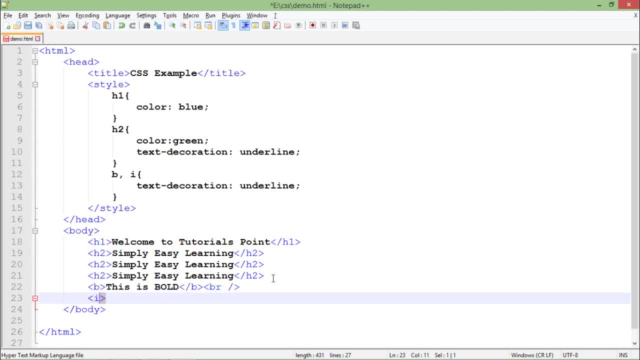 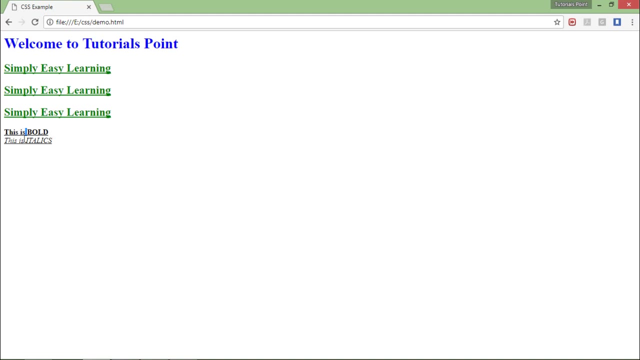 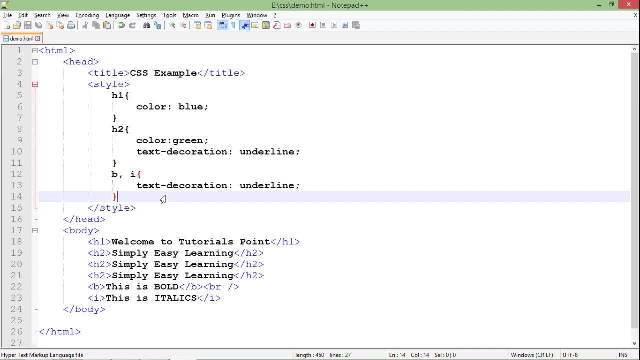 again, I'll put another I. that is italics, this is italics. all right, so here you can see. both are coming with the underlines, whether it's bold or italics. now you can also use the nesting here. by the time you want to work with any nested things, like for example for: 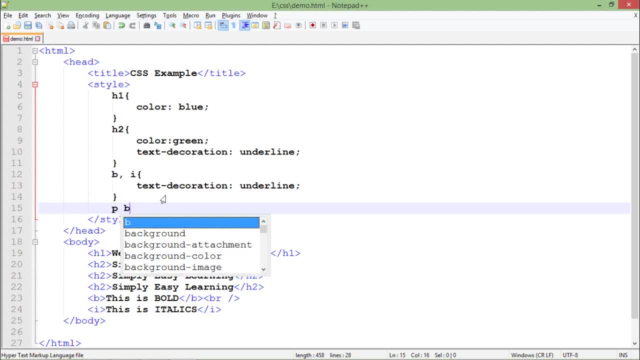 paragraph inside a paragraph, I will put a bold tag, and for bold, I want to do something like what I want to do. I want to say background color to lime green, all right, so what? it will mean that if I will put any bold tag, that will not be. 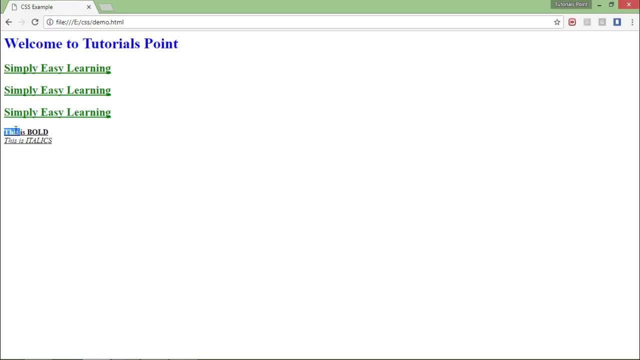 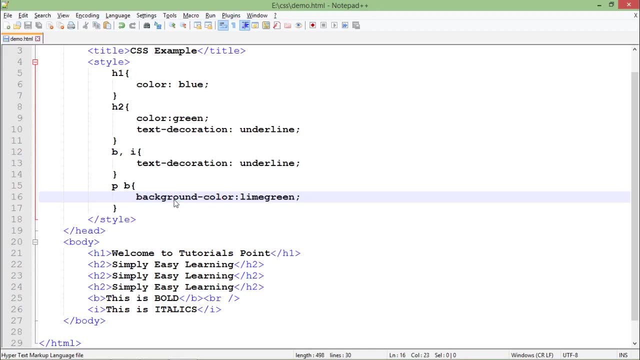 decorated with this lime green, as here already I have a bold, let me refresh it. but here you can see there is no background. this background color, lime green, is only applicable for those bold tags who will be there inside a paragraph. so let's see, let's start a paragraph this. 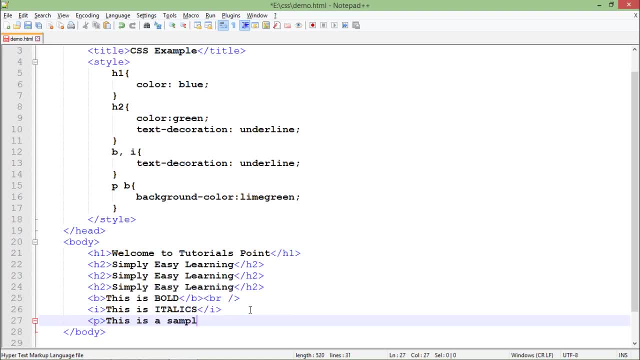 is a sample paragraph with a highlighted bold text. all right, so now here what I will do: I will start the bold tag here, I will finish it and then I will put a here. all right, so inside this paragraph I can see there is a bold tag. let me. 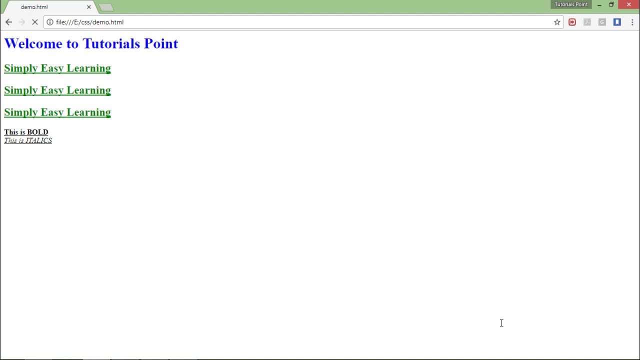 close the P tag also all right. so let's come here and refresh. and here you can see this is a sample paragraph with the highlighted bold text. and here you can see it is bold. it is underlined as well, because here I have designed the underline design for the bold text. all right, if you don't want to use underline. 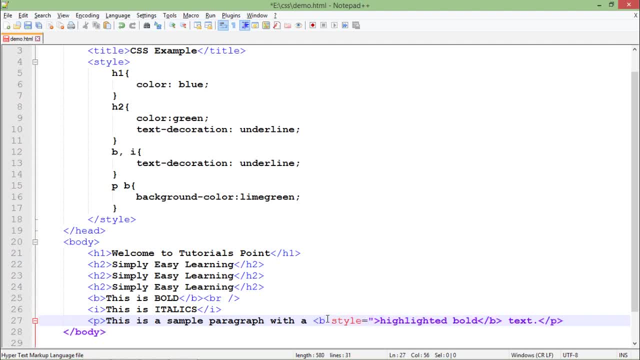 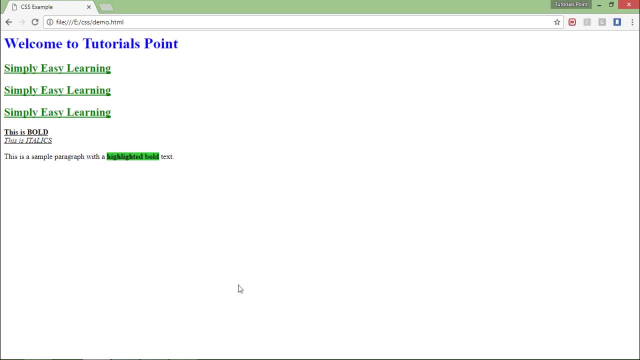 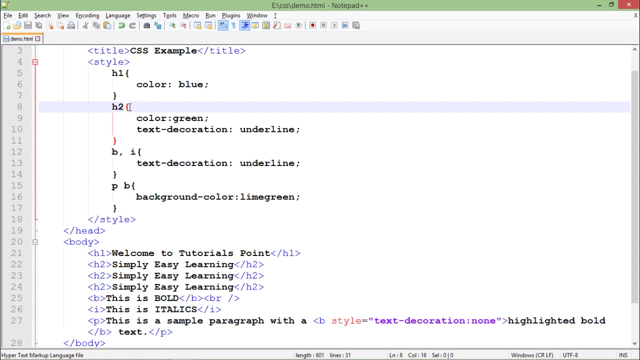 here. so again, you can come for inline style and you can use the text decoration to none. all right, so here you can see. for this there is no more underline. let me zoom it out, just make it clear. all right, so this is about the name selector. so you can use these names the way you want. now the another way to. 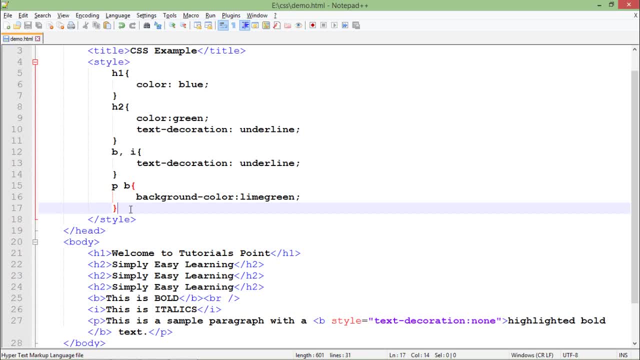 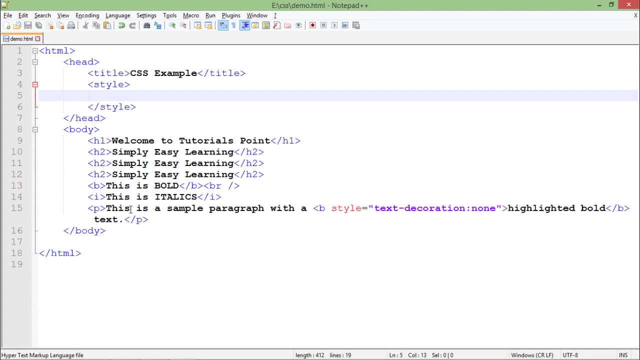 use the thing inside a CSS is the class selector. the reason why there is a Class selector concept? because there may be a situation where you want to put the similar styles for the different tags, for example. let me first remove this one. what I'll do for the class selector. first of all, I will use dot. that is a. 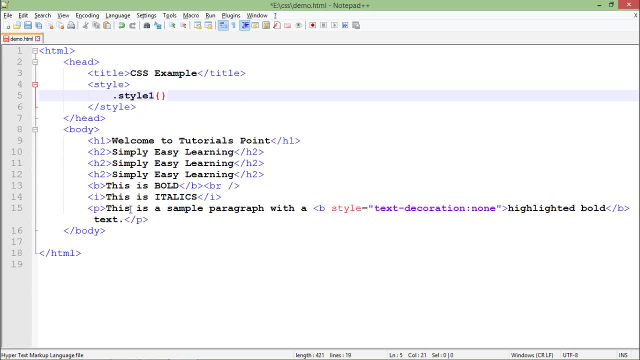 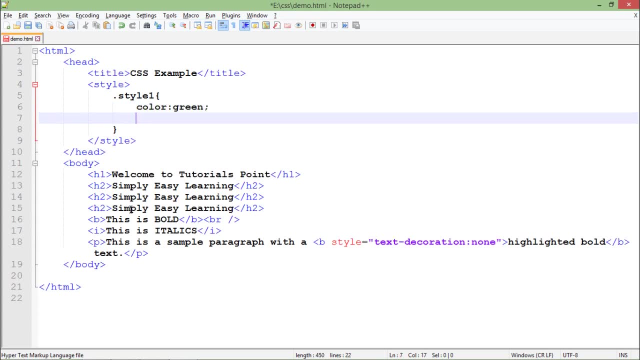 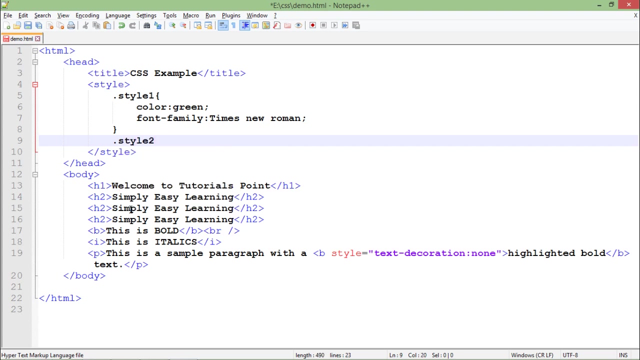 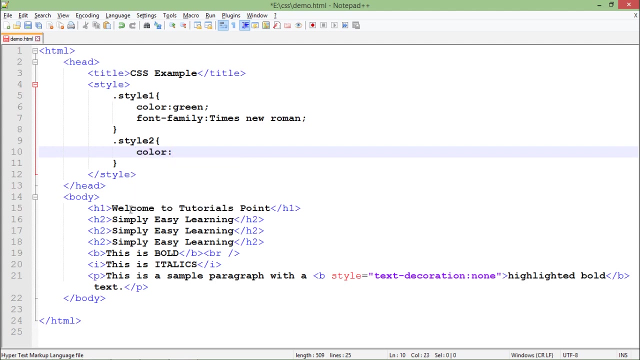 class, all right, and here I'll set different style class. let's say the first style: here I will use the color green and font times: new Roman. similarly, let's put another style style to another class, all right, and here I will use again, though, the same attributes with a different value, like it's red, and font family to monotype Corsiva. 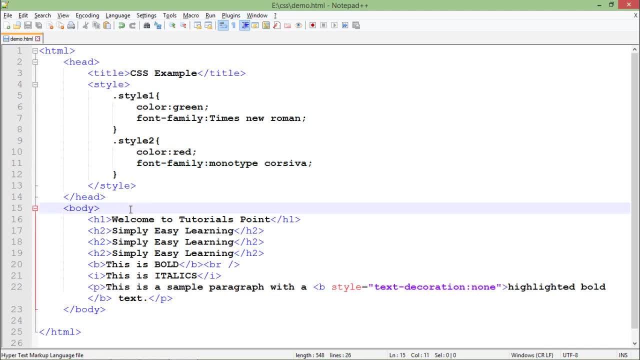 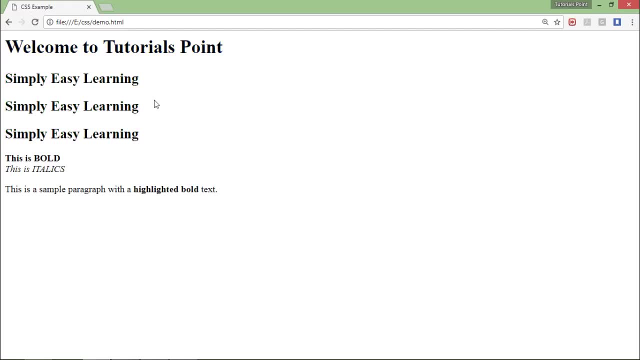 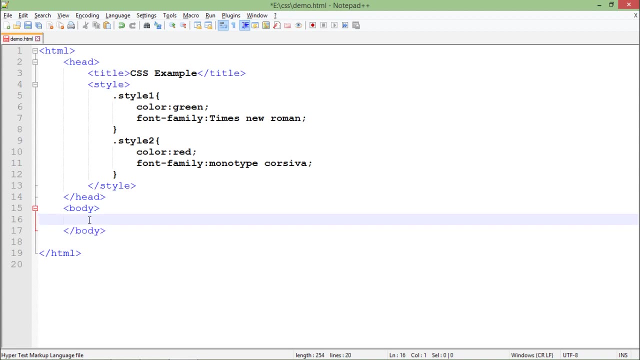 all right. so now here, I have not specified like for which particular tag I want to put these styles. I, if I am saving it, you can see all the styles are gone away, all right, so let's remove the text as well. I'll put some relevant text here. so what my requirement is like here. 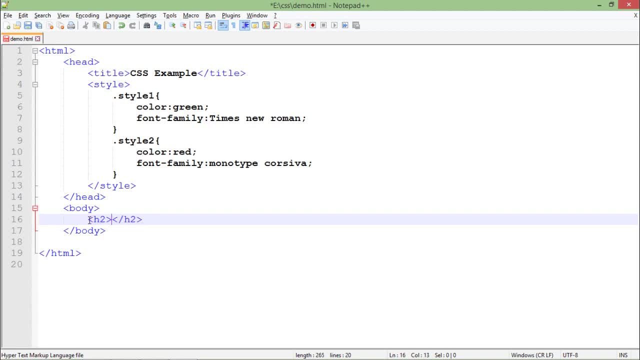 I am putting an h2 at the heading, like heading one, and for this particular heading I want to put a paragraph. so this is a paragraph for heading one. similarly, I want to put a paragraph, I want to repeat the same thing, for one more tag that is h2. again, it's heading two. this is the. 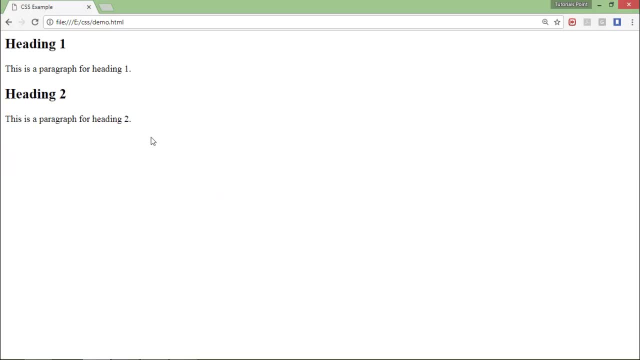 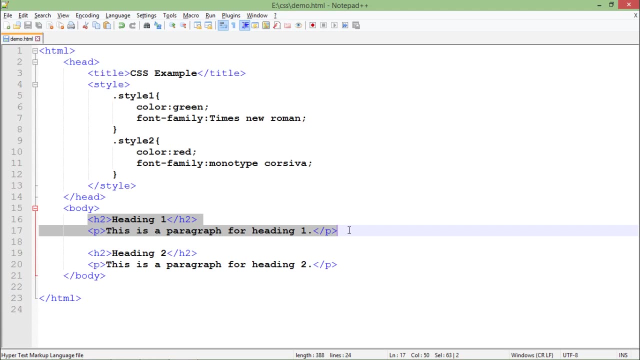 paragraph for heading two. all right, so now, this is the updated test. now what I want to do is I want that this heading and its relevant paragraph should come in a similar manner and this particular couple, like this heading and a paragraph, should come in a similar manner, but with the different styles. 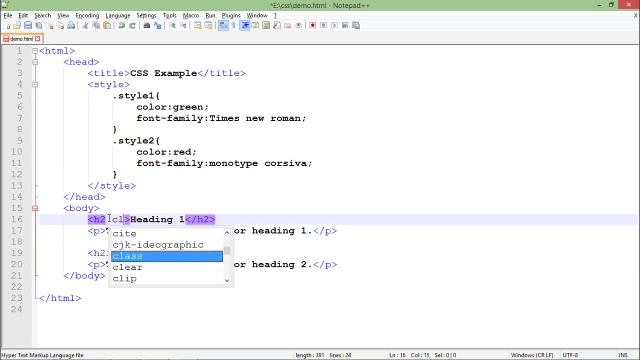 which I have already defined here. so what can I do is I will use the attribute class, and here I will pass the name of the class, like style one. all right, so let's close it now, all right, and I'll do the same thing. see, I use the 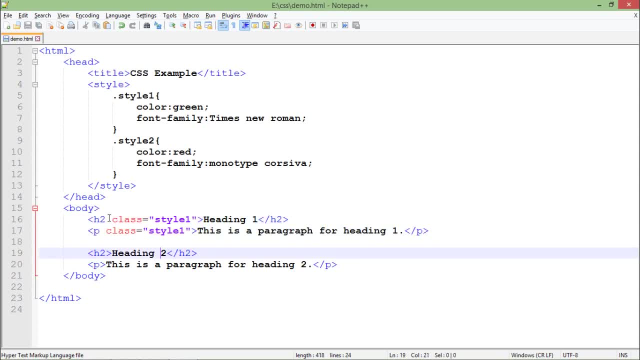 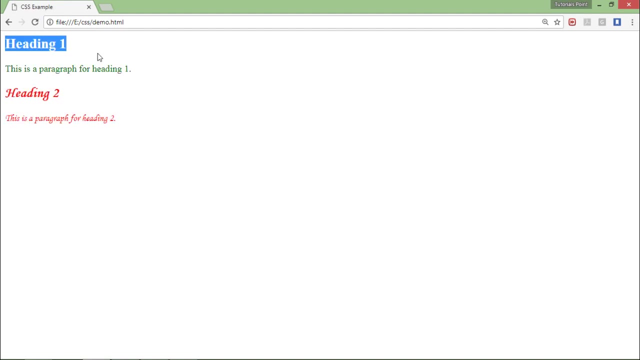 same style for this paragraph as well. similarly, in this particular situation, I will again use a class attribute with a different value. that is style two- and I will use the same class- that is style two- for this paragraph. so let's come here and refresh and you can see that both of these class, like h1 and h2- here means heading one and 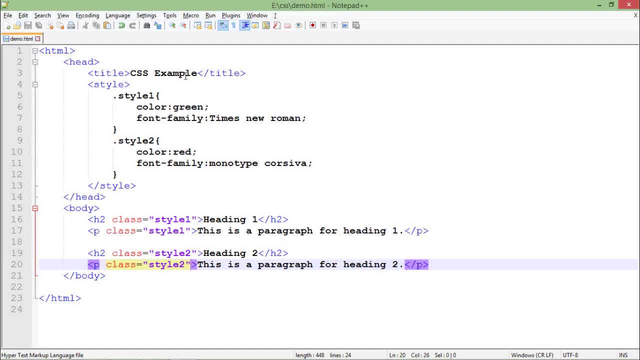 heading two are being decorated with the different classes of style. all right, now what I'll do is is I'll enclose them all inside a div. all right, I'll put it all inside a div. let's close this. for now it will not be reflected. but now let's add one more selector here, that is the ID selector. 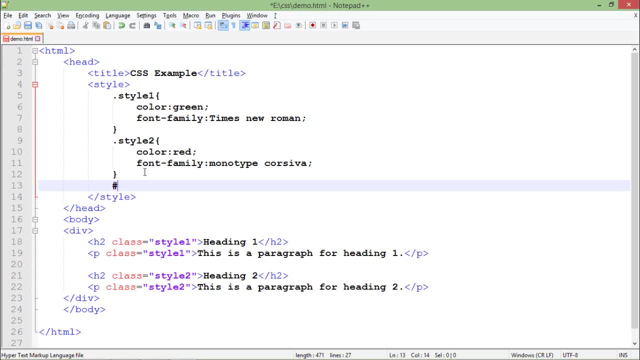 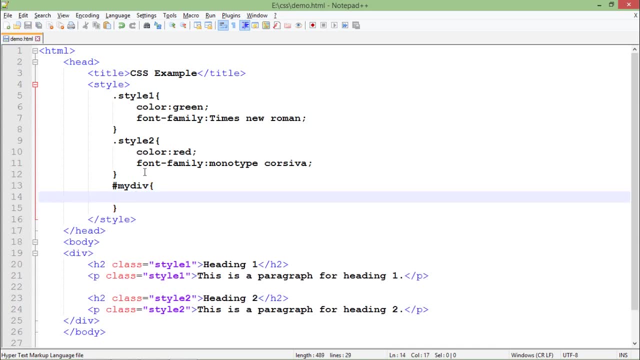 and for ID selector, I will use hash. all right, so like my div is the ID selector. ID is actually attribute in order to make a unique element in your HTML document. so what I'll do here: for making a div, I will use some of the attributes, like 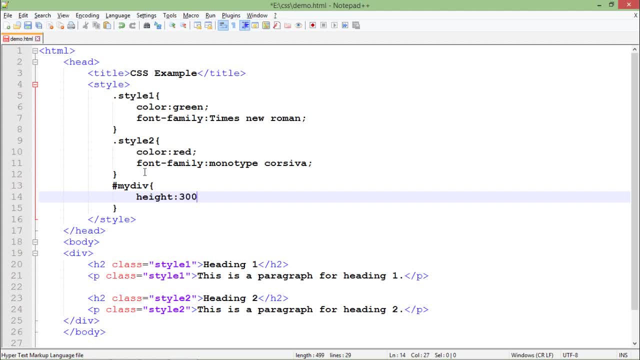 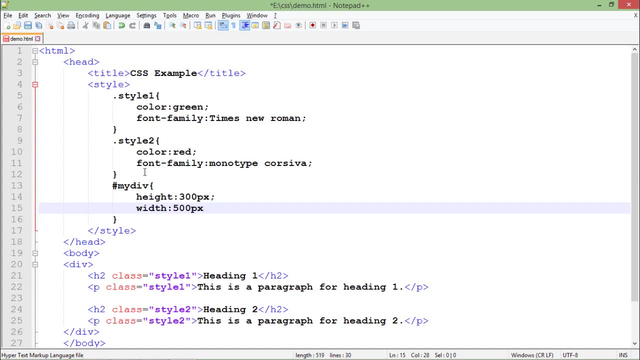 height. let's put height as 300 pixel, width as 500 pixel, all right. and we'll put a background color here, with the background color yellow, all right. now here's how I have decorated this, my div. but if I want to apply it here, what I'll do is I'll say ID.